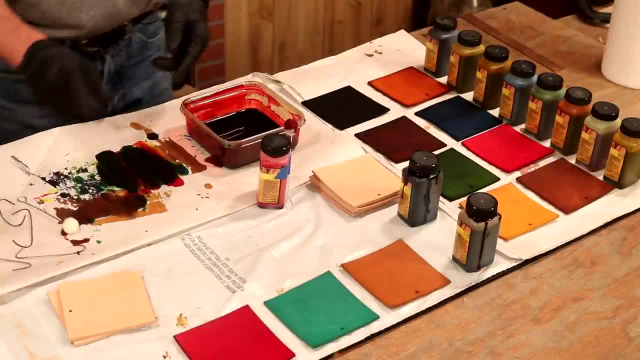 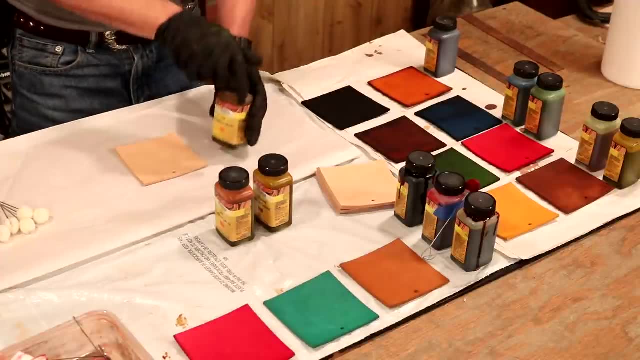 leather colors to our swatches with a couple of daubers. Let's see how that does. Let's start with our tan, because this is looking like it's going to be really pretty color. Now with our daubers, I'm going to go a little bit heavier. 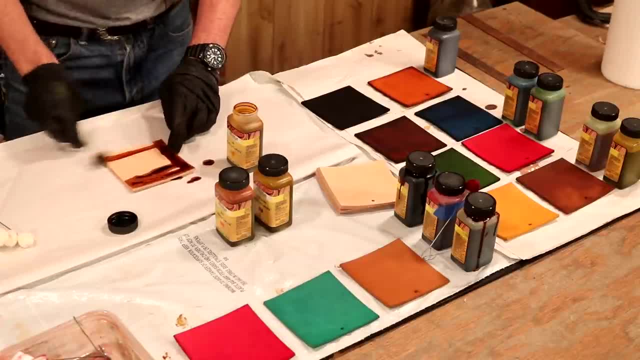 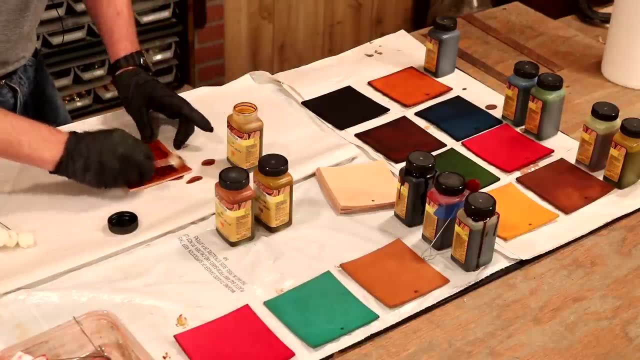 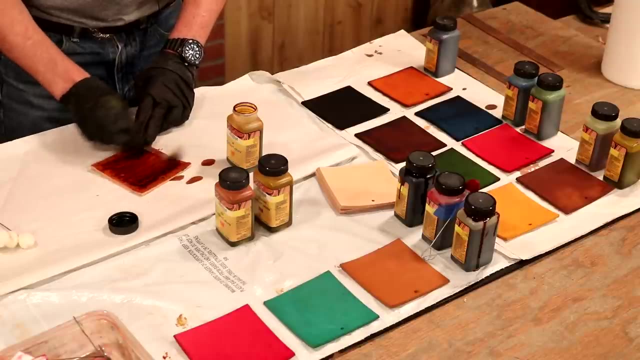 Let's get some full coverage on there, much like I would with a Pro-Dye: Get a good coat, Get as much as I can on a first good pass. Then let's come back in with a second pass, Now the water-based. it doesn't look like it wants to wick in, but all told, it seems to be. 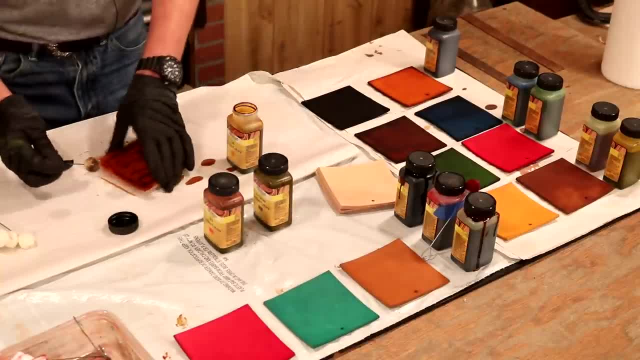 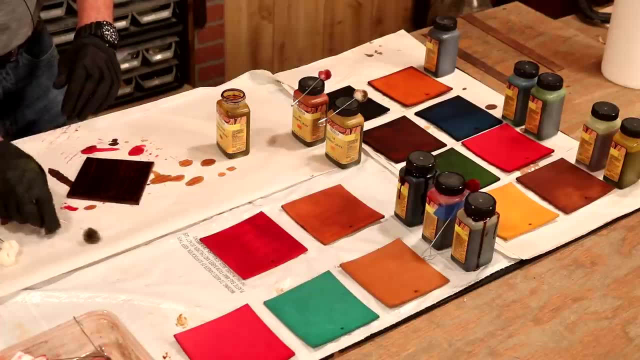 All right. so let's do the red, dark, brown. We'll see how this looks. Let's go kind of heavy on that. see how that's going to look. All right, I'm going to set this aside, probably give everything here, maybe four hours. 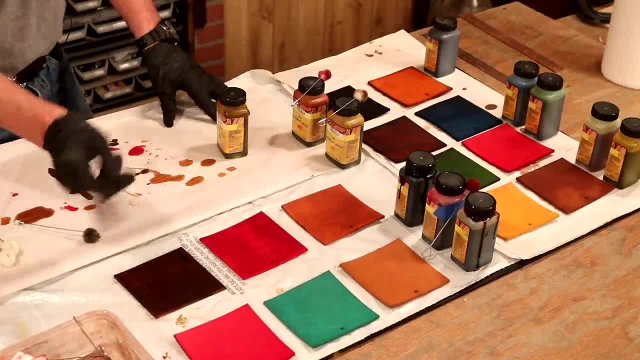 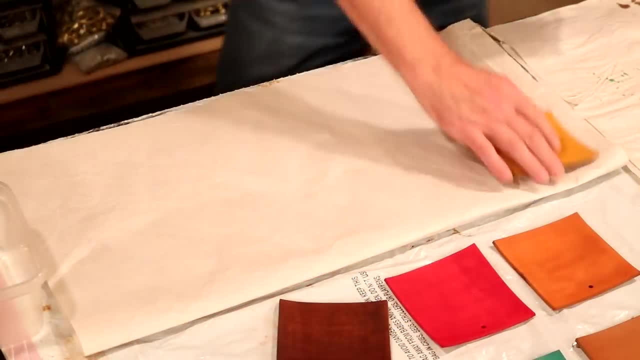 to dry. Let's see what it looks like Now. it's going to be flat. We're going to add a top coat here very shortly, but we'll get a good feel for the colors already. We've had some good dry time. 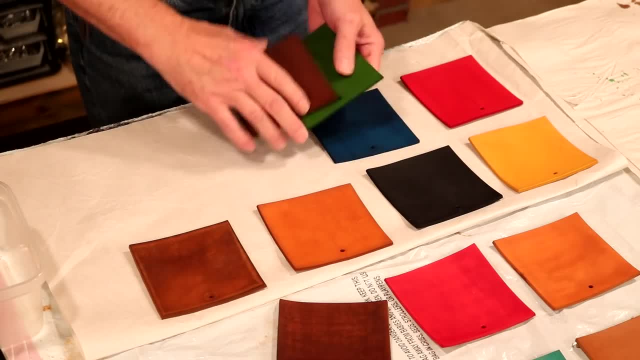 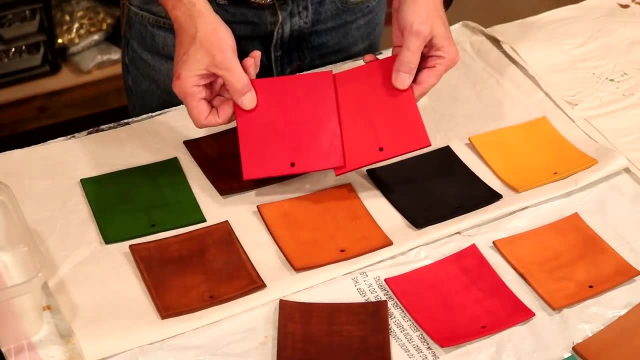 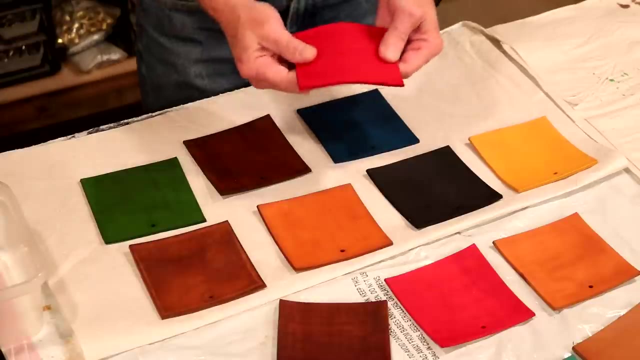 and, to be perfectly honest, some of these colors are absolutely beautiful. The green: it's a little bit more of a forest compared to the Pro-Dye. The red, though: look at that- absolutely identical, but look at the consistency on the two. That's part of what I'm looking for Now. stiff The. 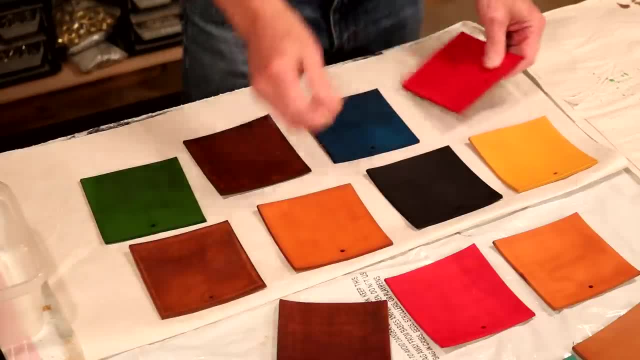 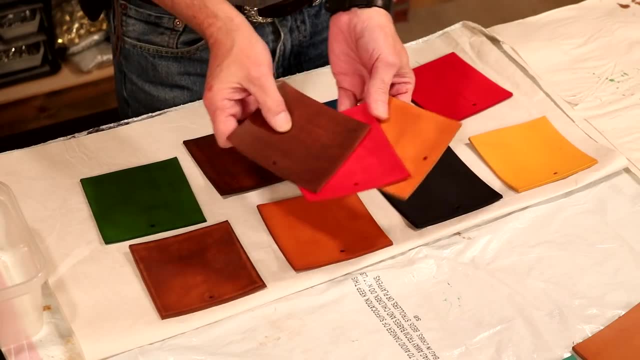 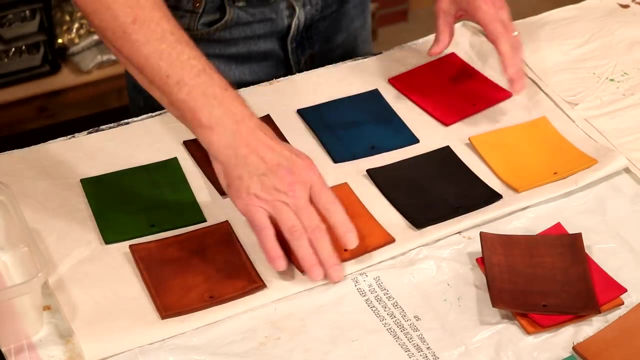 water-based very stiff. I assume these will soften up Oil-Dye still a little bit stiff, but not so bad. Now the three that we've done with the Dauber- I could be happier. They're streaky, not very consistent. So all told, dip-dyeing easy way to go. 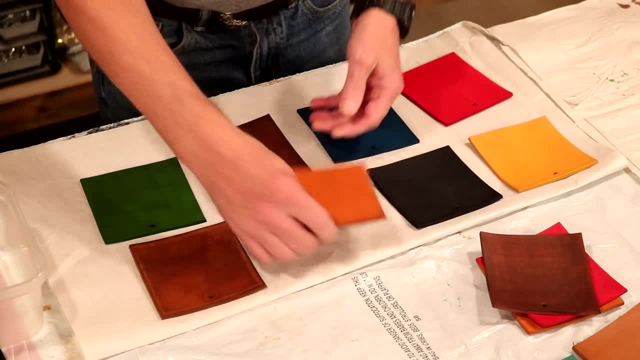 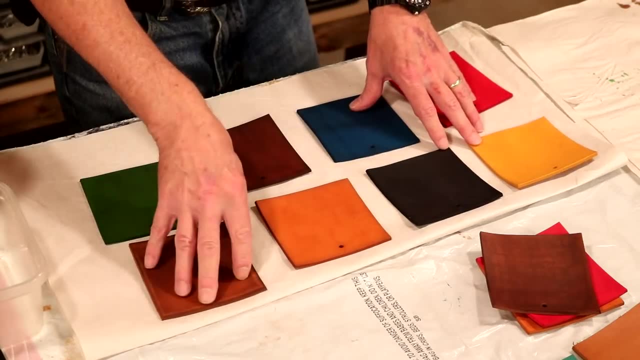 Right there, that is our tan. That's a beautiful color, So let's do this. I'm going to add some leather balm. We're going to put a top coat on all of these. We'll look at these on a gray background. 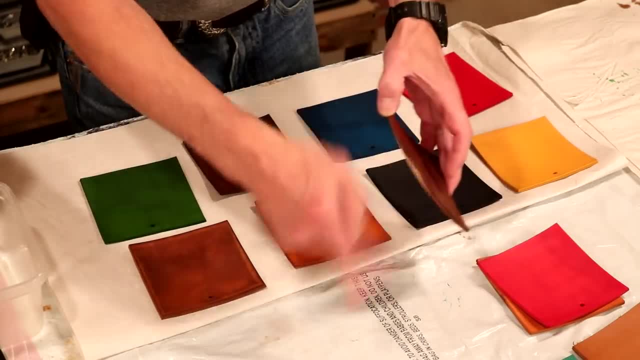 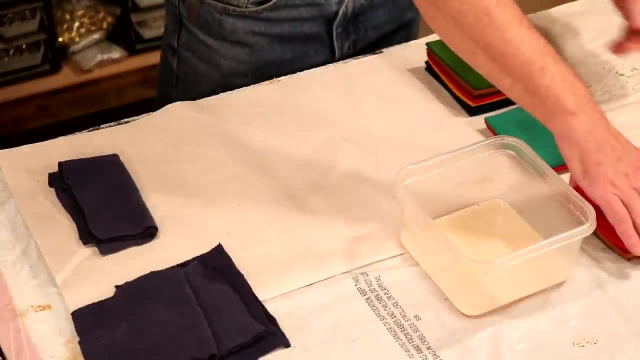 so we can get a good feel for the color. Our last step: we're going to cut some of these open. Let's see if that dye's wicked in as well as I hope it has. So we've got our three stacks. This is our. 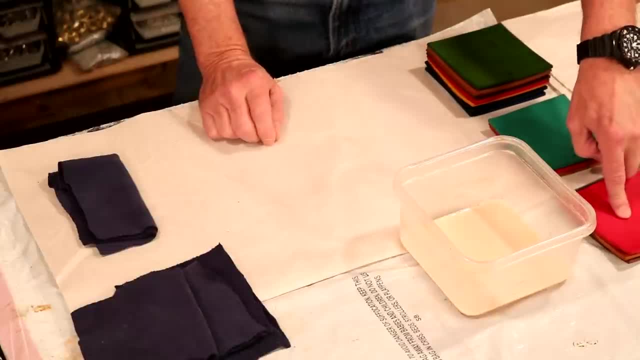 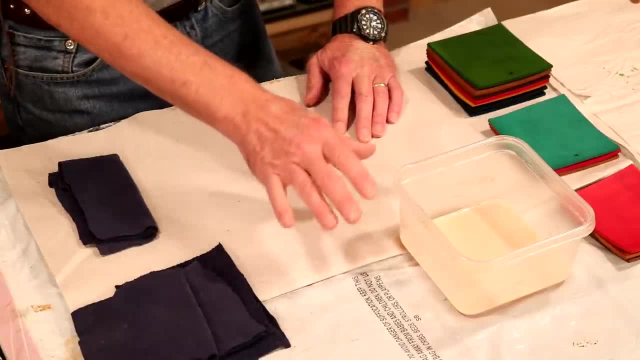 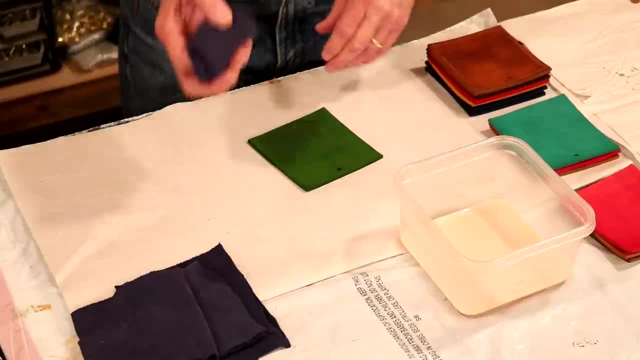 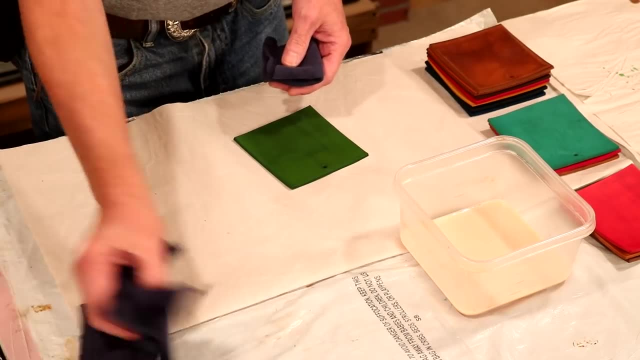 color. So to apply this, what we're going to do for the test here is I'm going to use a different rag to apply for each, so I don't transfer color over. Then I've got some dry rags here that I'll. 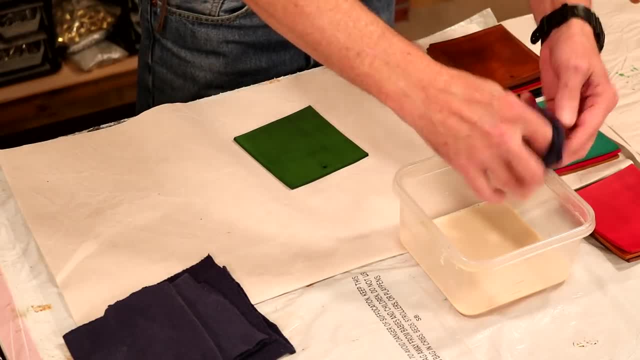 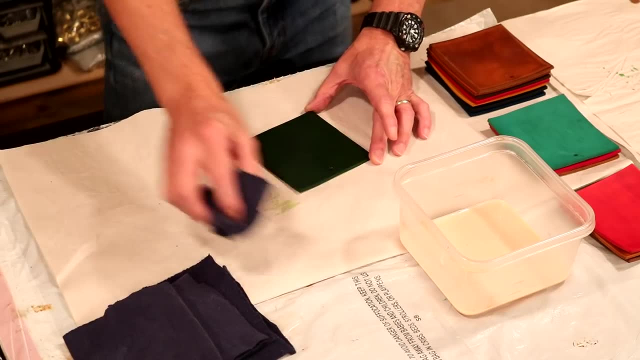 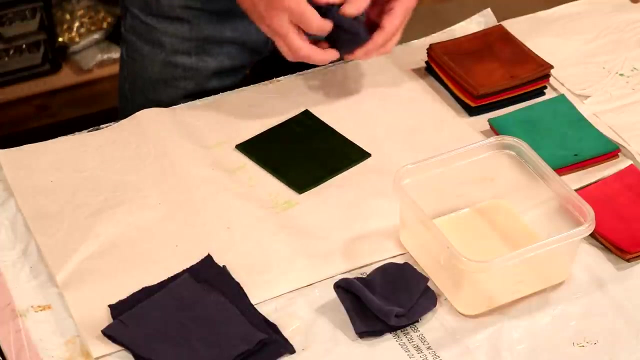 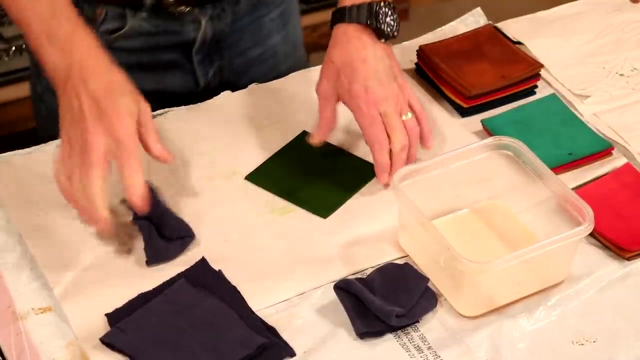 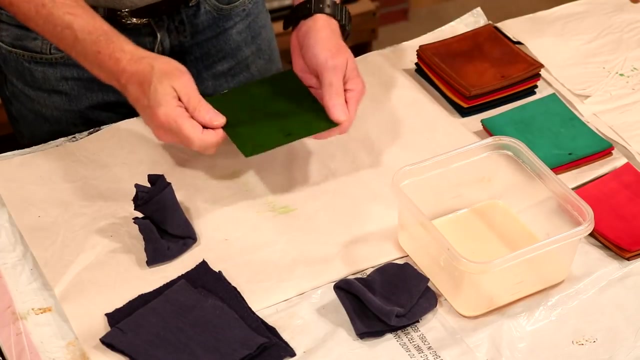 buff with And a little buffing. Well, that actually looks pretty nice. We'll get a closer look here in a minute, So I'm going to add the leather balm to the rest of our swatches. Then we'll get a good look at these. 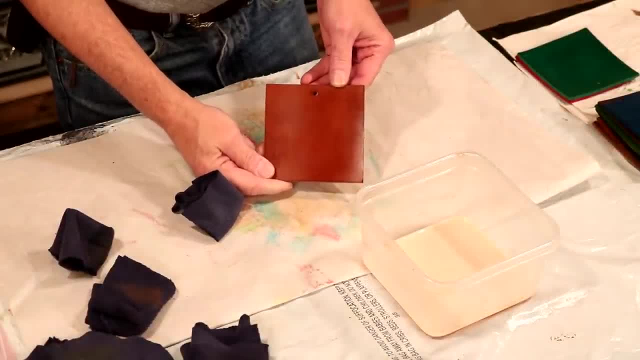 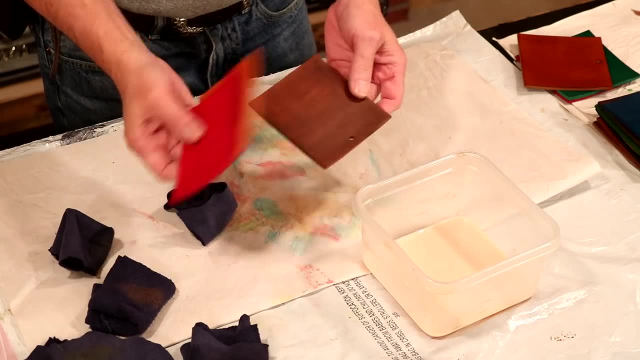 Last one. Look at that. Doesn't that look good? Beautiful pro dye, I love it. Okay, I'm not going to go to the trouble to put top coat on our Dauber Applied. We already know what we need to know there, So let's step over to our pattern table. I'm going to lay out some good. 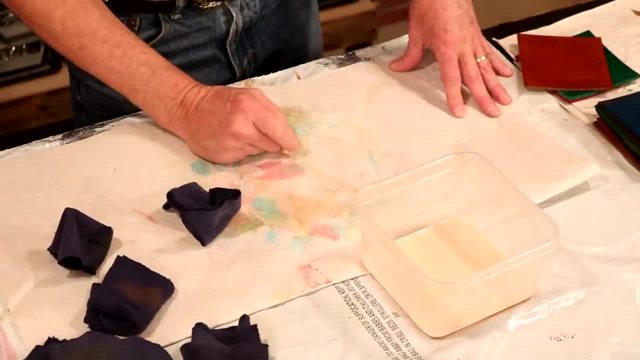 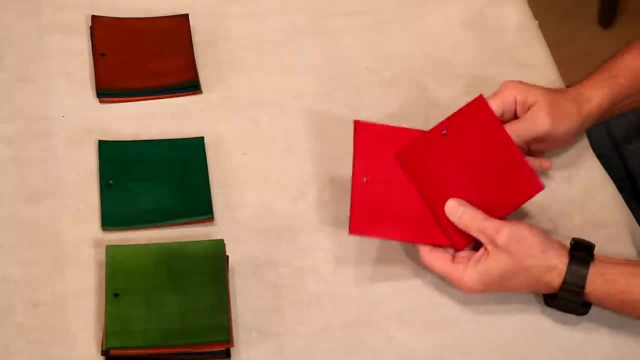 gray, suede. dump some light on that table. Let's look at some comparisons. So with this let's start. right here, our reds, Those are beautiful. So right there, we've got our pro dye and our water-based, our leather color- Both good colors. 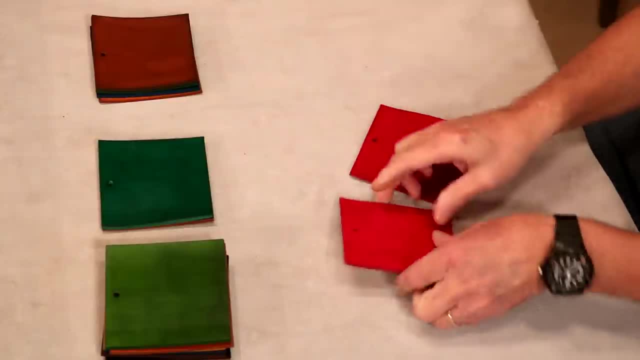 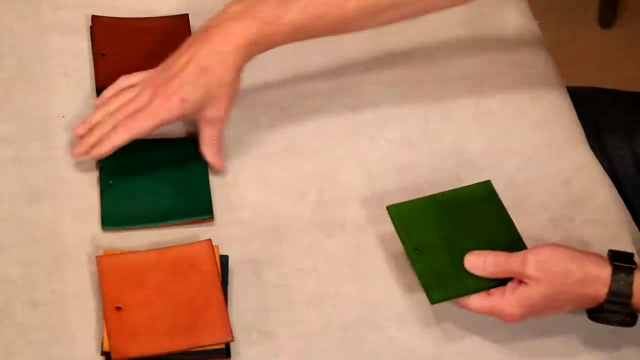 This is a little bit more rich, A little bit softer too. The water-based, that's pretty stiff, but nonetheless we could work that out, We could soften that a little bit. The greens- well, they're both pretty greens, Happy with both of those. A little bit more stiff, a little bit. 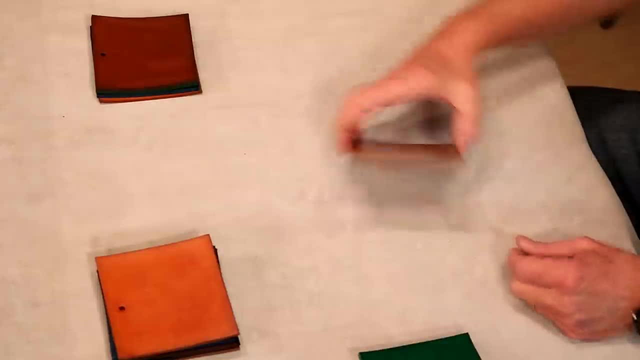 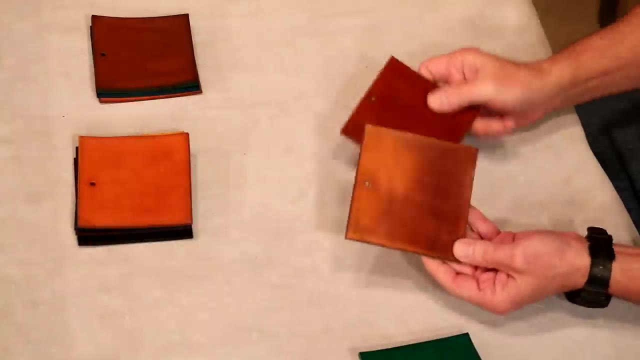 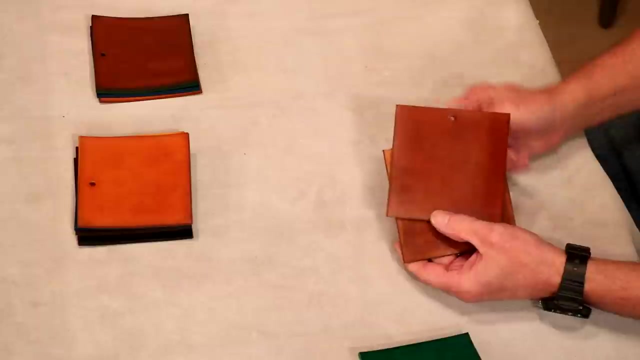 softer. Now let's jump over here. Let's see, Right here, that's our light brown pro dye. look for our medium brown, because I really wasn't very happy with that. Now, not to say that we can't add maybe another coat or two to get that a little more consistent, but, all told, look at the pro dye. 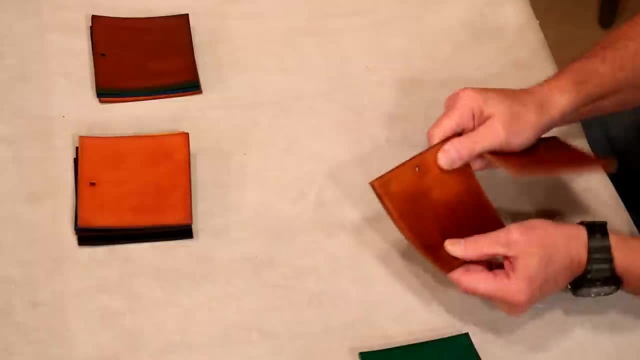 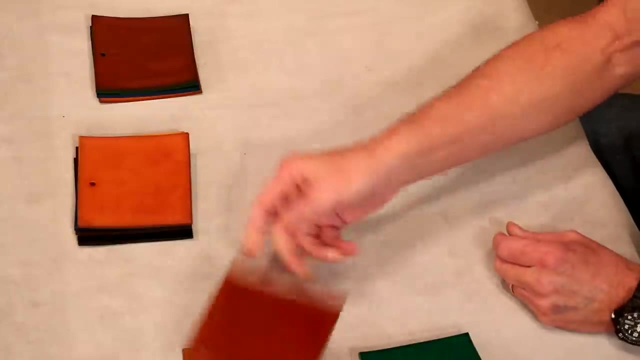 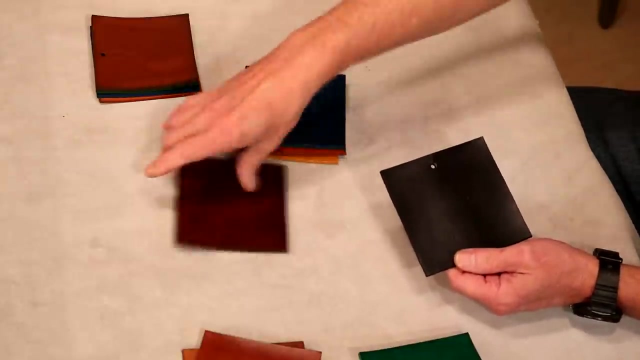 the difference there and again. actually that's not terribly stiff, so we might just not have gotten enough dye on that A little bit more stiff. but boy isn't that beautiful. Now over here, nice rich black, that looks good, and our dark brown love that color. that came out nicely. So all told, I'm pretty. 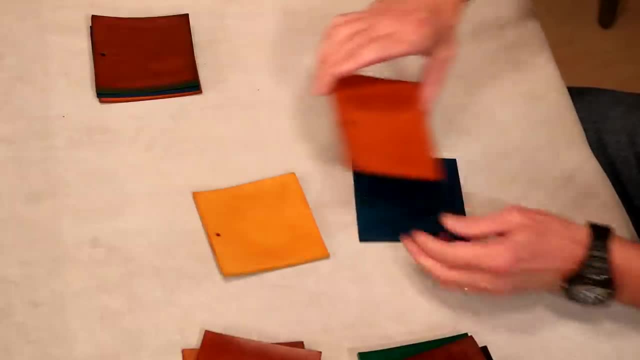 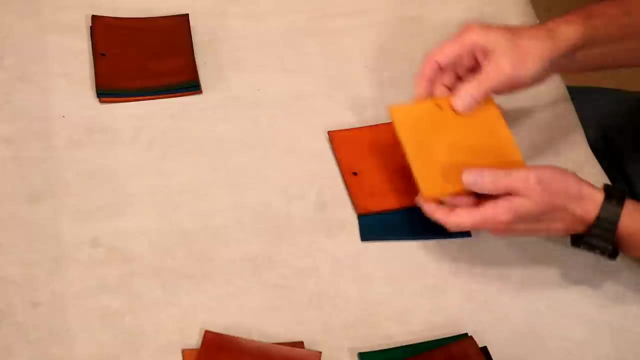 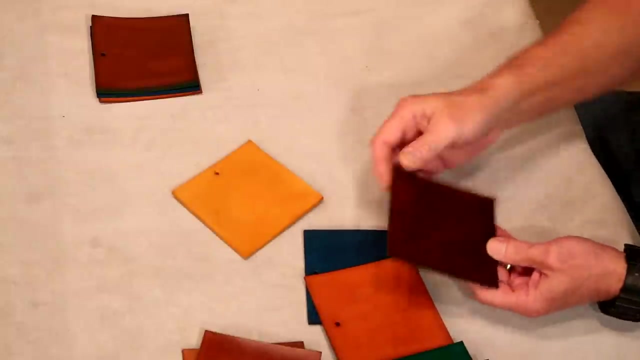 happy with the water-based colors. There's our blue- let's see, I believe that's our tan- and then the yellow: Good crisp colors, but consistent too. Now one last point. we're going to step back over to the table. cut some of these open. but one last point. I tend to say that the the leather balm is. 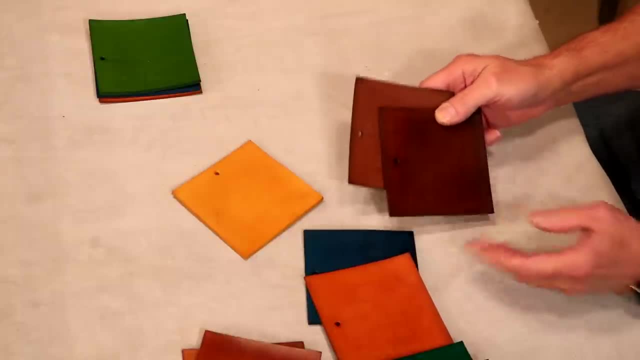 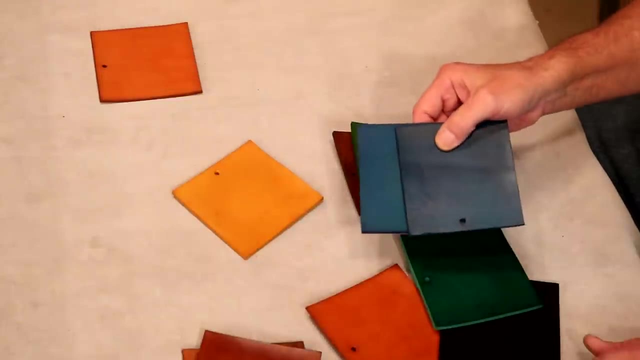 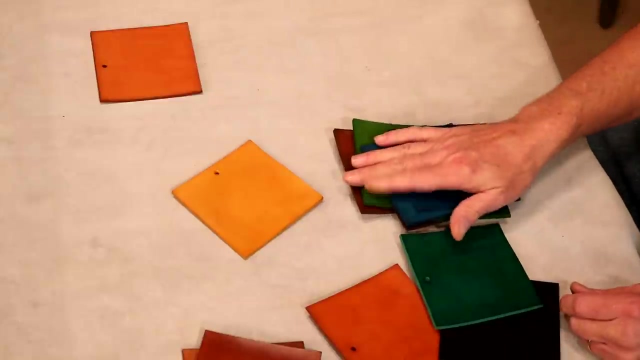 going to darken, But all told it does darken a little bit, but it's really not bad. In fact there's the green and let's see there's our blue. So all told it does enrich in the dark, in the color, doesn't necessarily darken it once it starts to dry off. Okay, let's step back to our main table. let's cut. 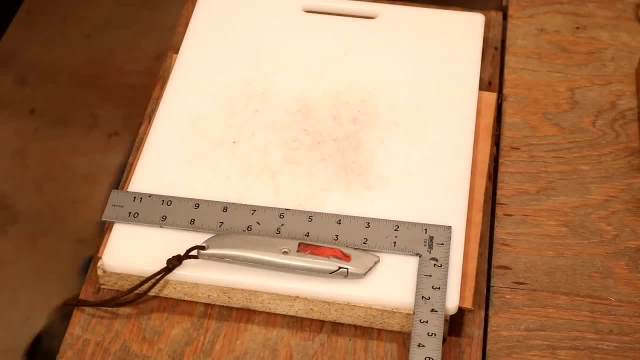 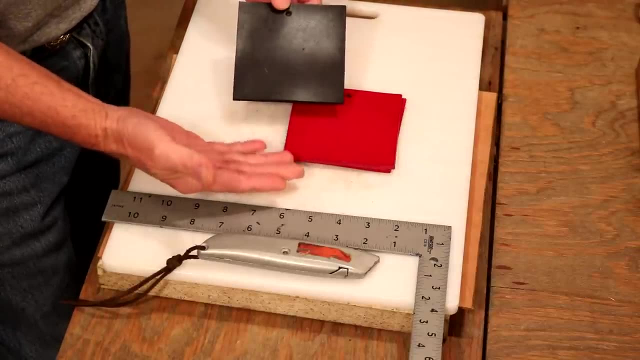 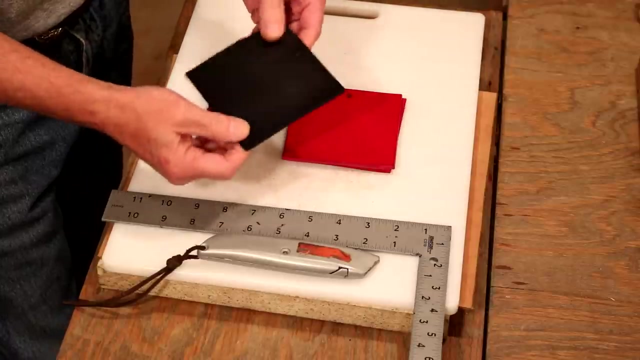 a couple of these open. see what we find. One of the reasons I've been hesitant to use a water-based dye is its ability to wick in. In my opinion, alcohol is going to wick much easier than water. But all told, look at that black. that is a gorgeous black. looks good with a top coat. Now it's a little. 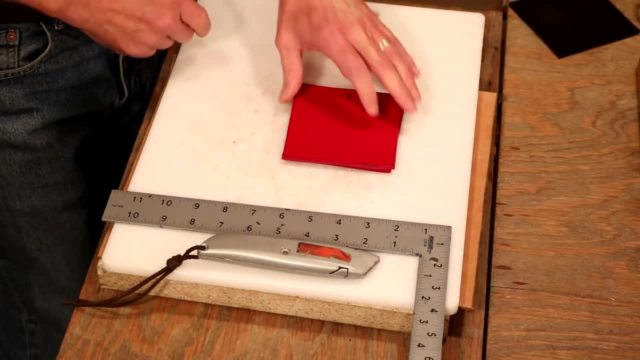 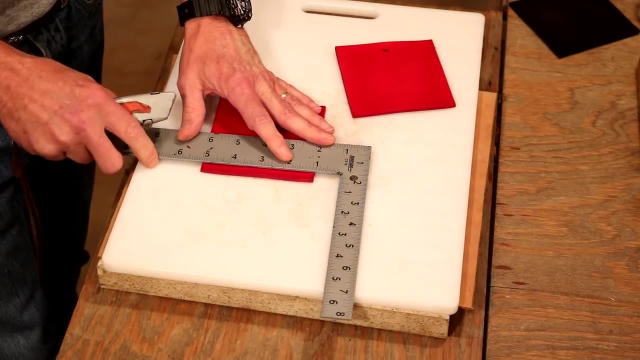 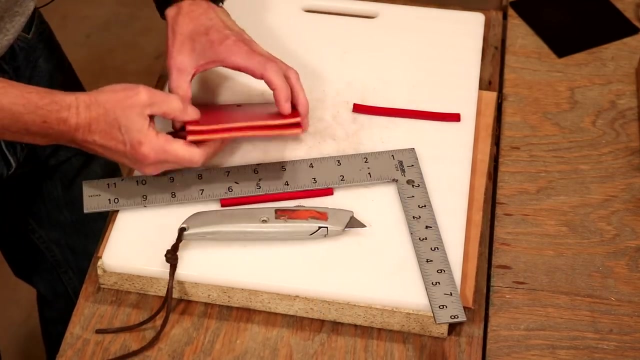 bit stiff. we can deal with that. That looks good. So let's do this. I've got our leather colors. let's see that's our pro and our leather colors. Let's cut these open and see what happens. Okay, pro on top, leather color on the bottom. let's get a little better. look at that. 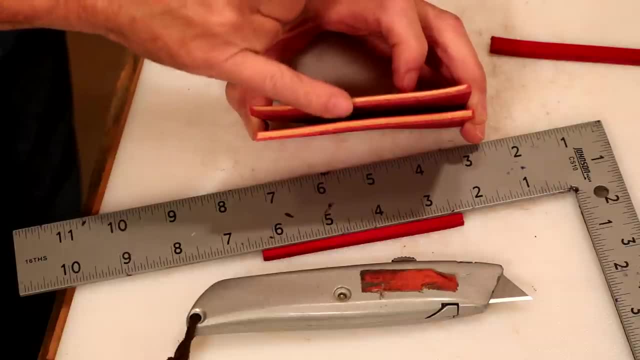 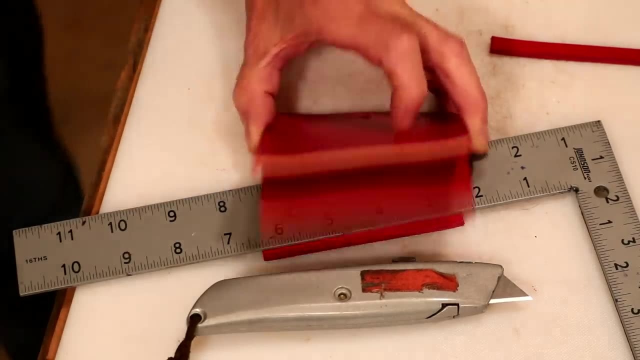 Our pro has wicked in a little bit deeper, Particularly on our flesh side, but all told, they both look good. I'm going to have to change my thinking on the leather colors, and that's exactly right. I think I'm going to have to reassess how I 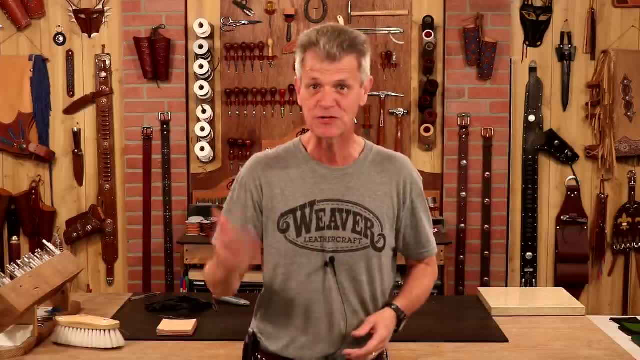 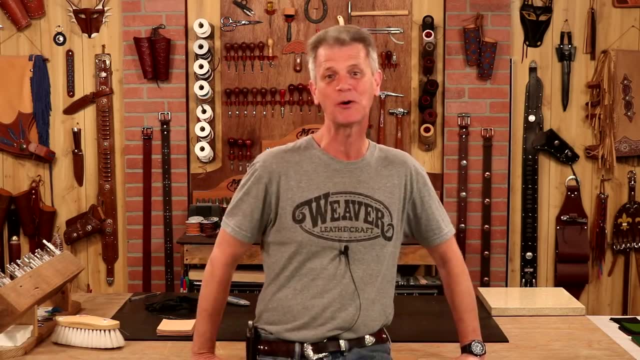 think about the water-based dyes. They look pretty good other than stiff. I see no other issues. I hope this is good information for you. Thanks for taking time to watch the leather element. Good luck with your projects.